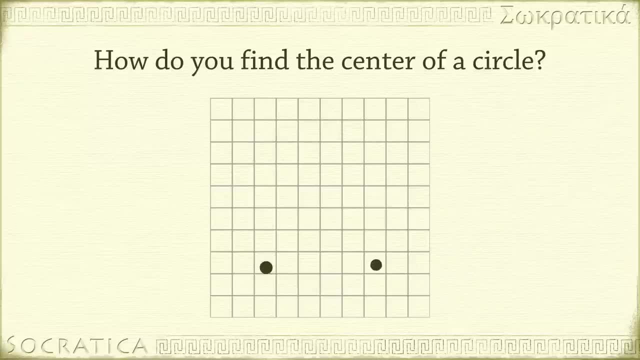 number of circles through that one point. If you have just two points, there are still an infinite number of circles through the pair of points. But if you have three points and they're not on the same line, then there is one and only one circle that passes through. 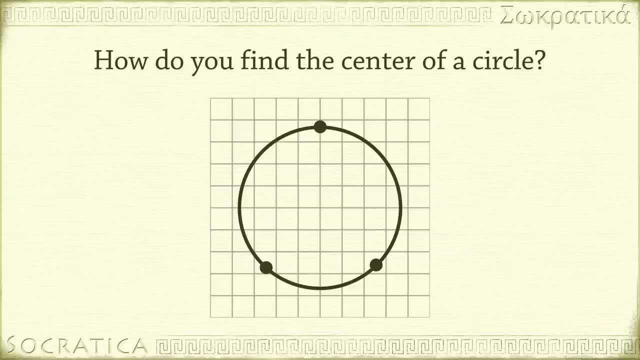 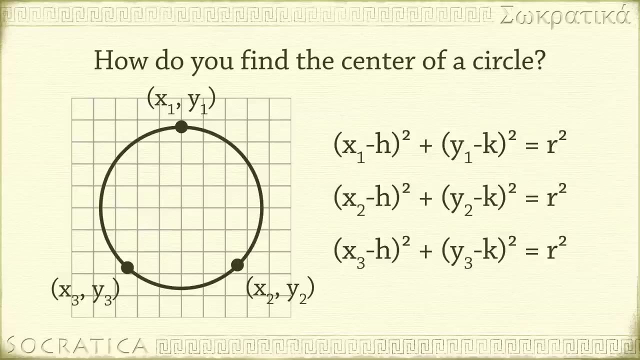 all three points. In this case, you can find the center of the circle by solving the following for h, k and r: To do this, plug the coordinates for each of the three points into the equation of a circle. You now have a system of three equations with three unknowns: h, k and r. Remember. 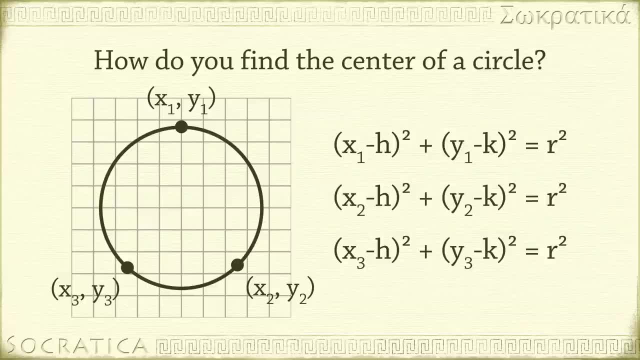 x1, y1, x2, y2, and x3, y3 are not variables, they're numbers. Once you solve this system of equations for the unknown parameters h, k and r, then you've found the center of the circle. 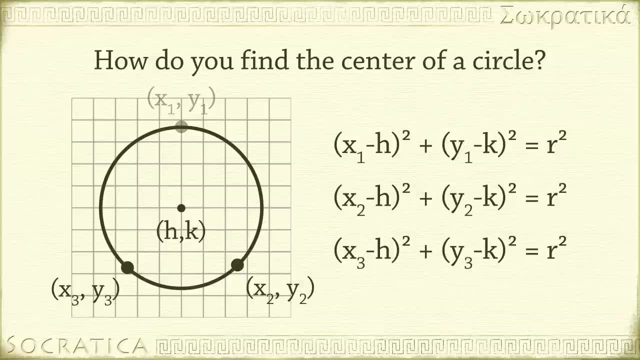 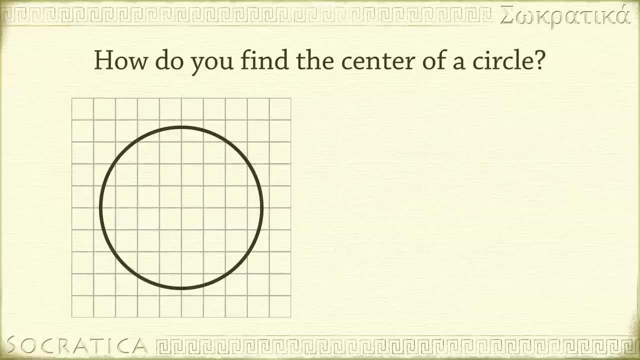 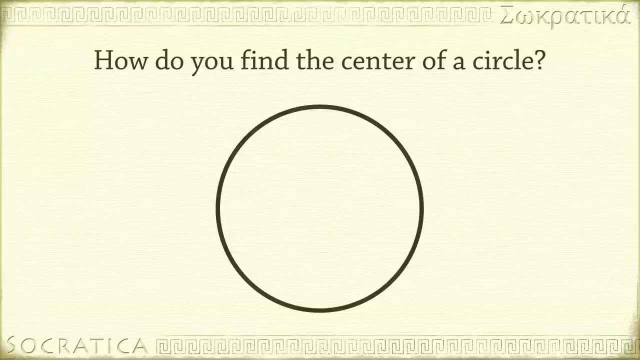 But here we only have a circle. We don't know the coordinates of any point on the circle. This may seem like a pretty hopeless situation, and it is, if you try to use analytic geometry to find the center of the circle. But you can do it using Euclidean geometry, And here's how. 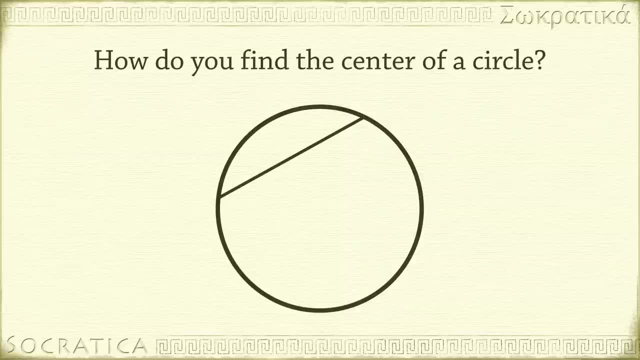 First draw a chord on the circle. Any chord will do. Now suppose we did know the center of the circle. Then if we connect the two endpoints of the chord with the center, we'd get an isosceles term. 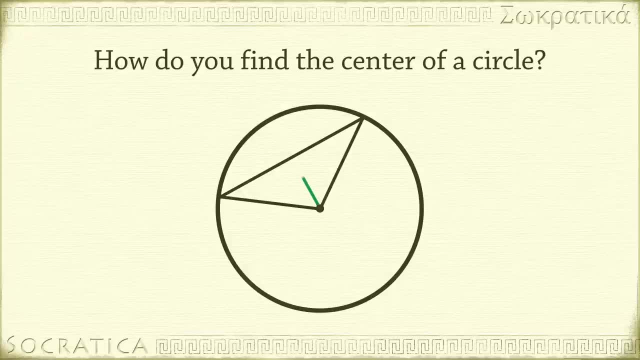 And this is the isosceles triangle. Now look what happens. if we draw an altitude for this triangle through the center of the circle, The altitude cuts the isosceles triangle into two right triangles. Both of these right triangles have the same hypotenuse r, and these legs are: 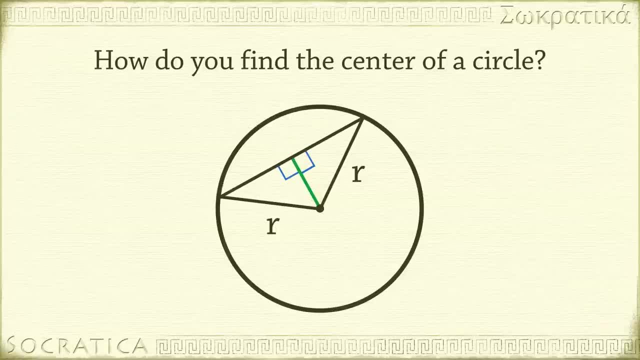 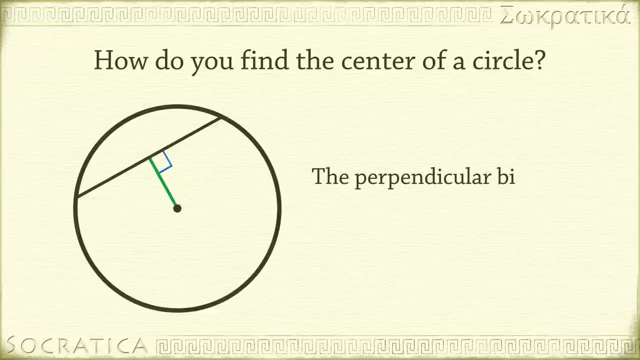 identical. So by the Pythagorean theorem the other legs are equal to each other. This means the altitude is a perpendicular bisector of the chord. In other words, the perpendicular bisector of a chord passes through the center of a circle. 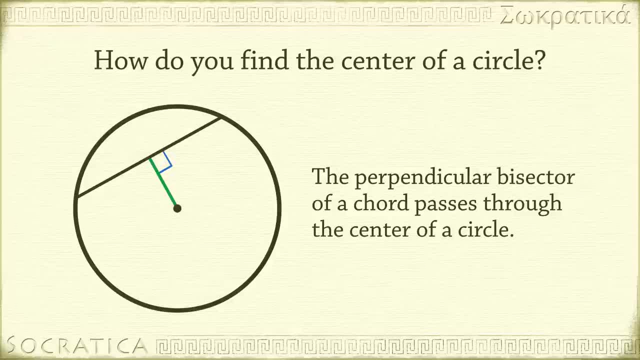 It's this fact that will allow us to find the center of the circle. Now, constructing the perpendicular bisector of a line segment is a classic geometric construction. If you don't know how to do this, or if you've forgotten, then check out our video on how to. 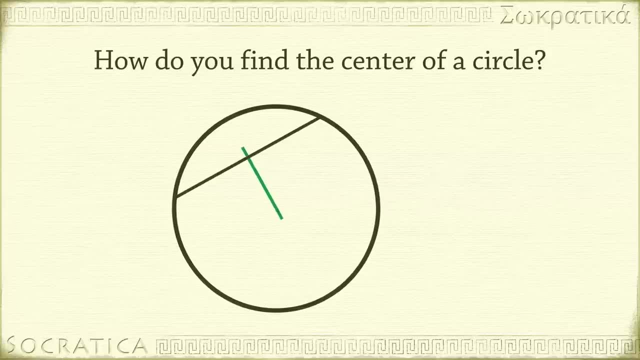 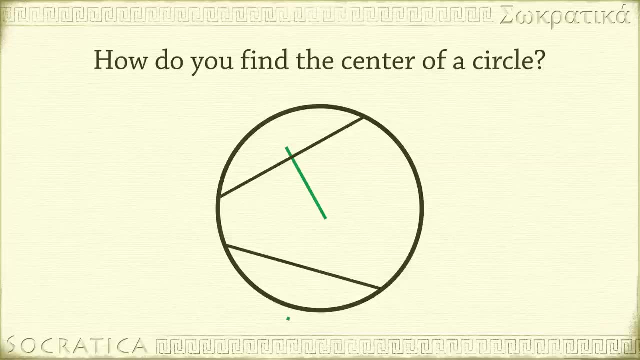 bisect line segments. We're now ready to find the center of this circle. To do this, we draw a second chord. Next, construct the perpendicular bisector of this new chord, Since each perpendicular bisector passes through the center. the perpendicular bisector passes through the center.